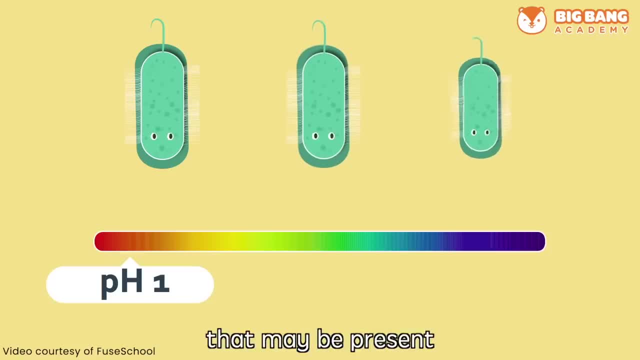 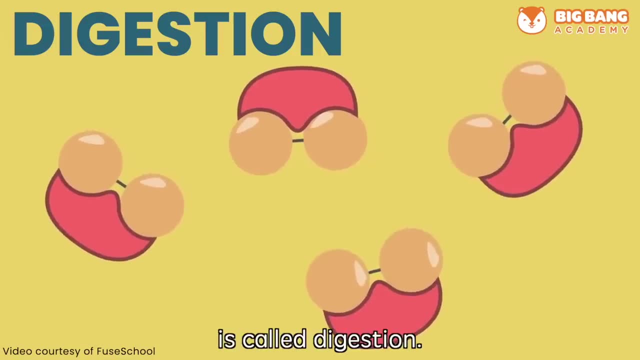 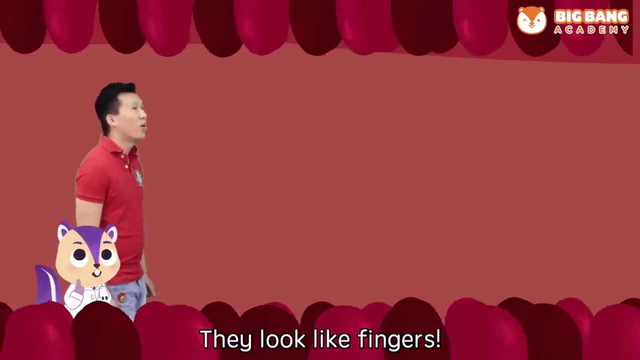 chemically and kills most of the germs that may be present in our food. The second step of food processing, in which we break down food into smaller pieces, is digestion. Whoa, Wow, what are those Nixon? They look like fingers. 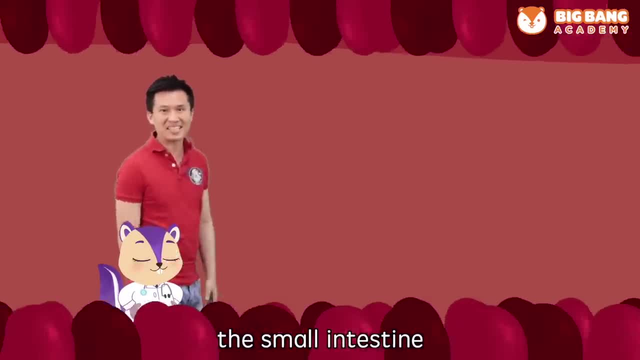 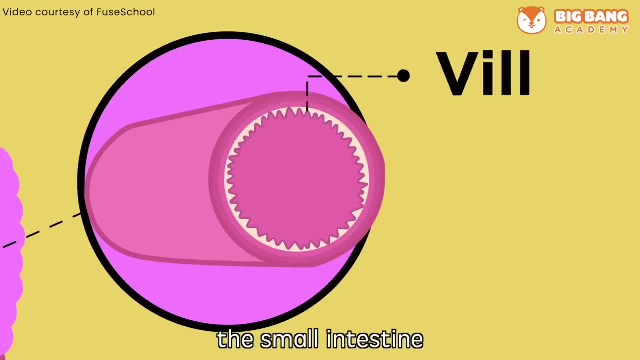 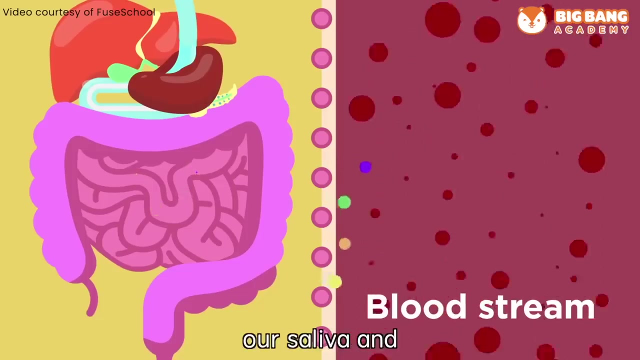 Yes, Bobo, we are now in the small intestine and those finger-like projections are called villi. The main role of the small intestine is to absorb the nutrients from our food that are digested by the enzymes in our saliva and the stomach just before. 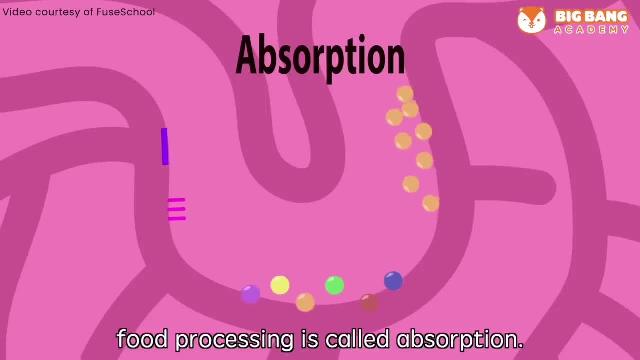 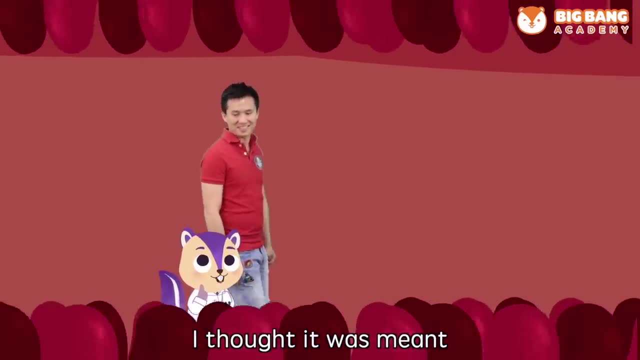 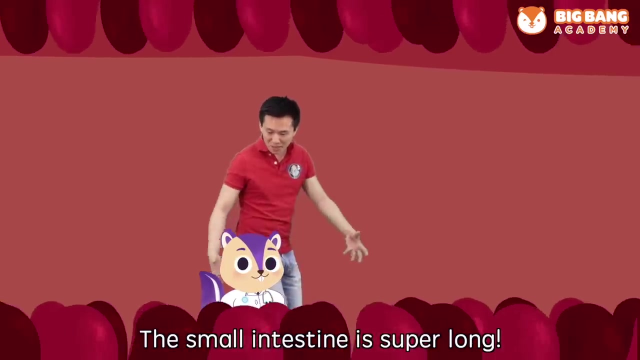 The third step of food processing is called absorption. Hold on a second. how long have we been in the small intestine for? I thought it was meant to be the small intestine. Yes, Bobo, the small intestine is super long. It's around 7 meters long and it's looped and packed in a very confined space. 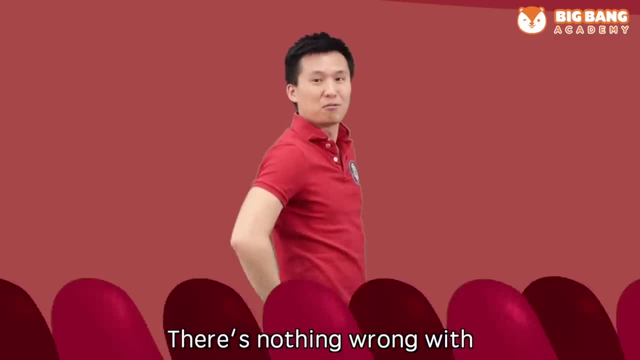 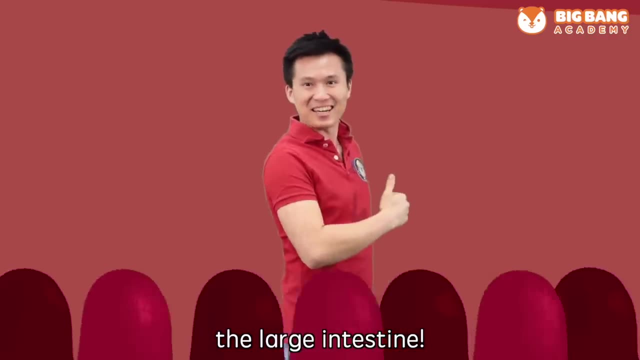 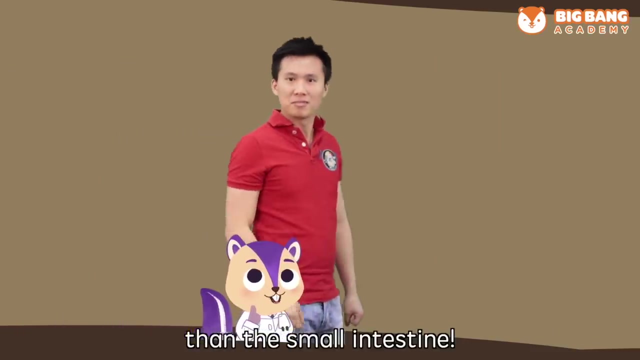 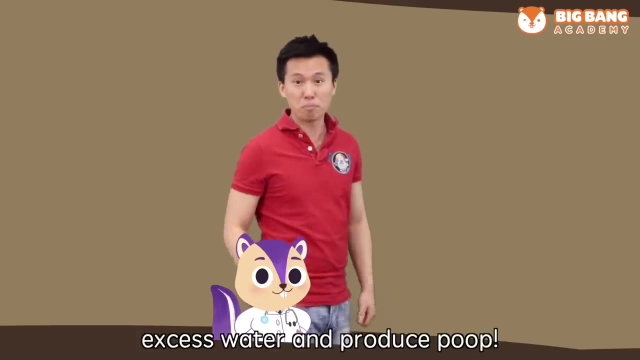 Look, we are here. We are almost at the end. There's nothing wrong with Michael's small intestine. Let's get to the next stop, the large intestine. Whoa, the large intestine is a lot wider than the small intestine. Great observation, Bobo. The large intestine mainly absorbs excess water and produce poop. 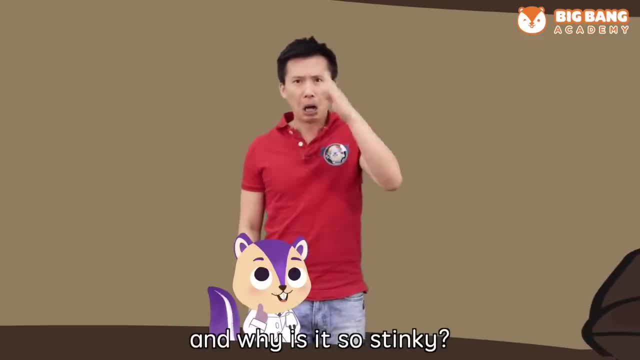 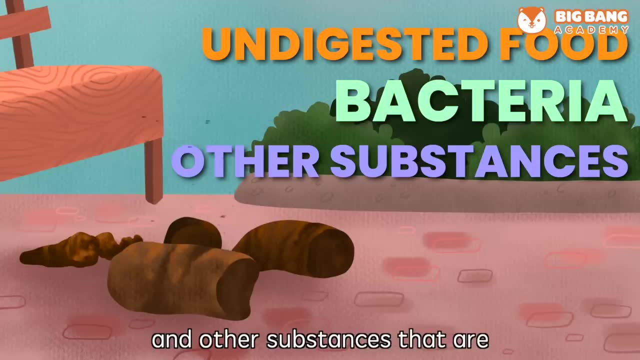 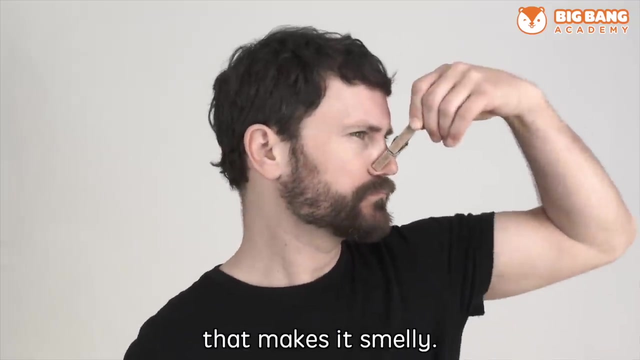 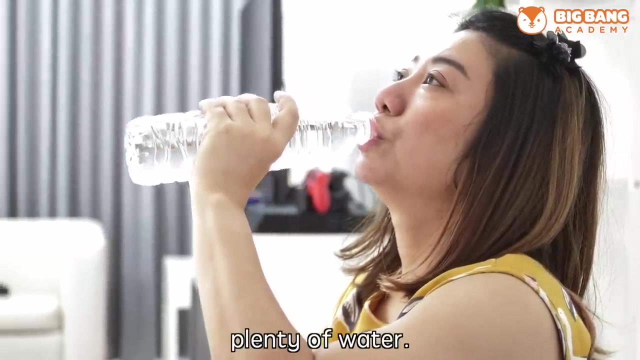 What's in the poop and why is it so stinky? Poop is mostly undigested food, bacteria and other substances that are released by the intestines. Usually, it is the bacteria in the poop that makes it smelly. An important way to ensure your digestive system stays healthy is by drinking plenty of water. 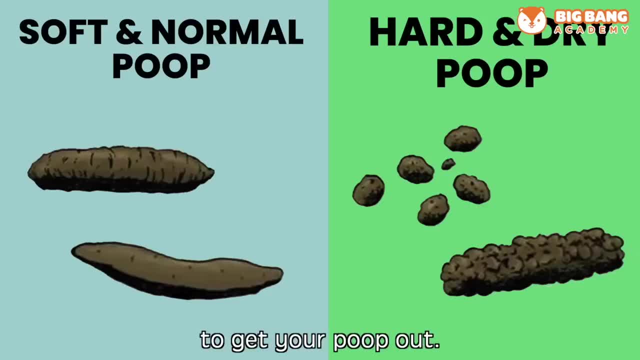 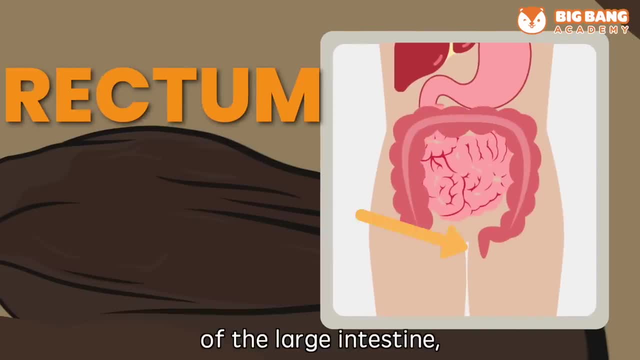 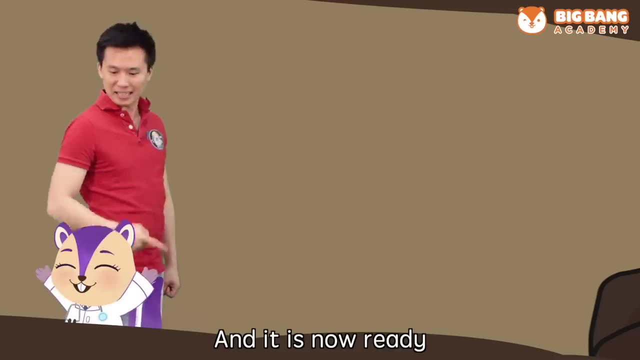 If you don't drink enough water, it would be much harder to get your poop out. And then we poop- Not yet Bobo. The poop is stored in the lower end of the large intestine called the rectum. Look at how the excess water is absorbed from the biscuit and it is now ready to be adjusted from the body. 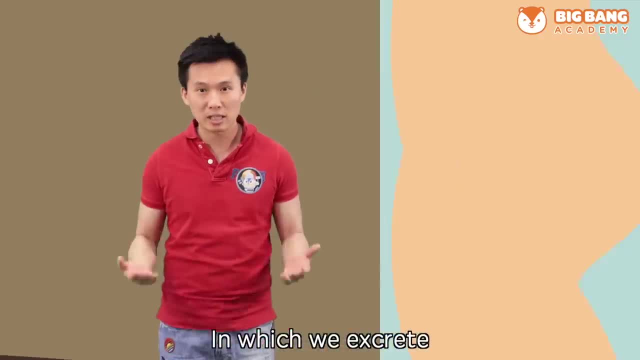 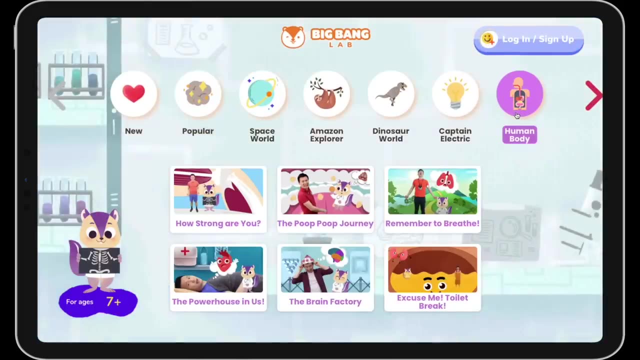 The final step of food processing which we excrete poop from our body is called elimination. Thanks for watching. Want to explore more of the human body with Bobo? Sign up now and get started with a free trial. See you soon.